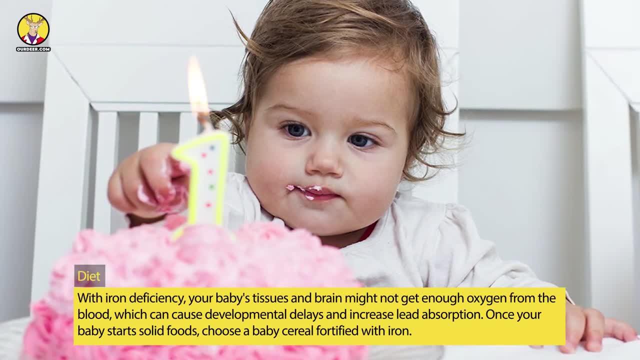 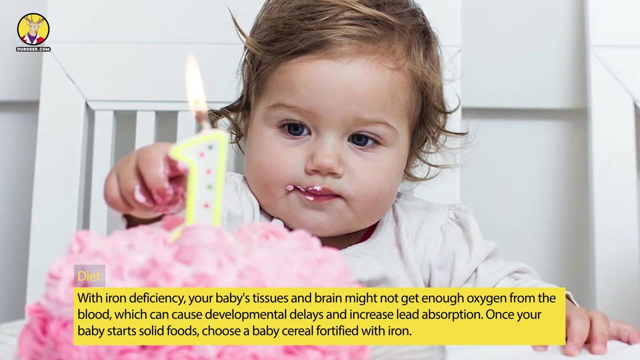 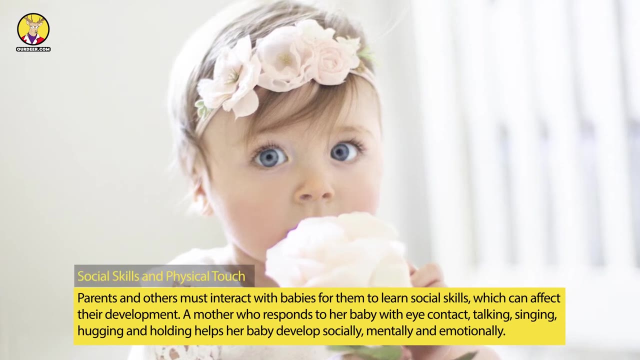 With iron deficiency, your baby's tissues and brain might not get enough oxygen from the blood, which can cause developmental delays and increase lean absorption. Once your baby starts solid foods, choose a baby cereal fortified with iron. Social Skills and Physical Touch. Social Skills and Physical Touch. 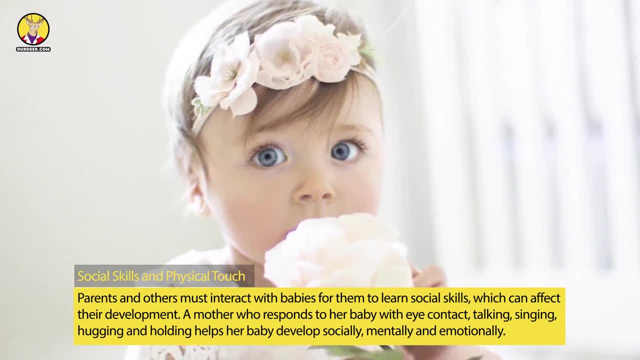 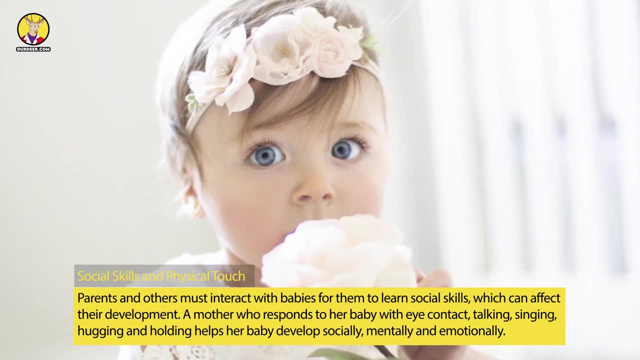 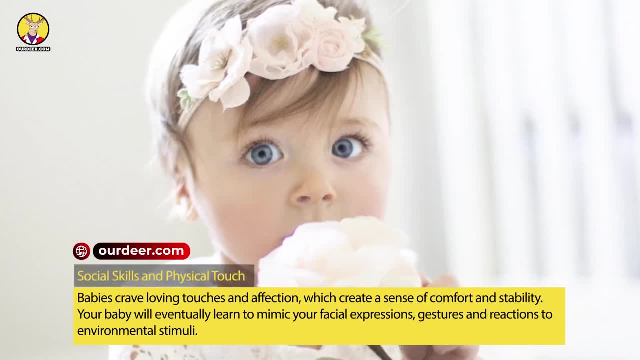 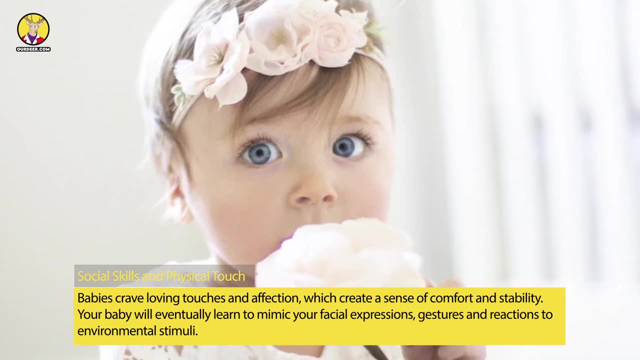 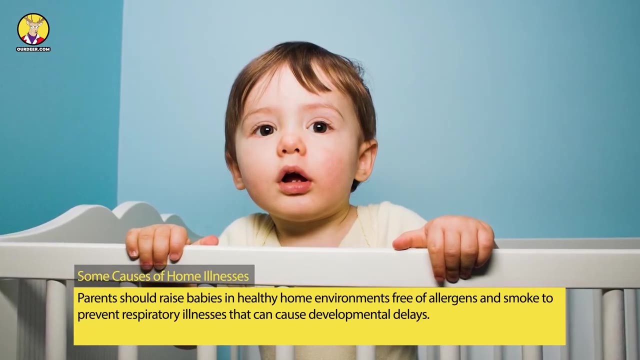 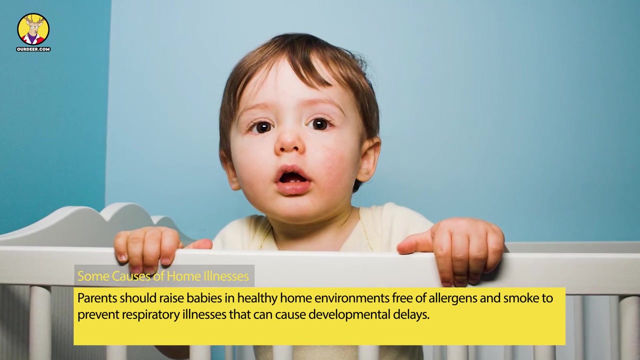 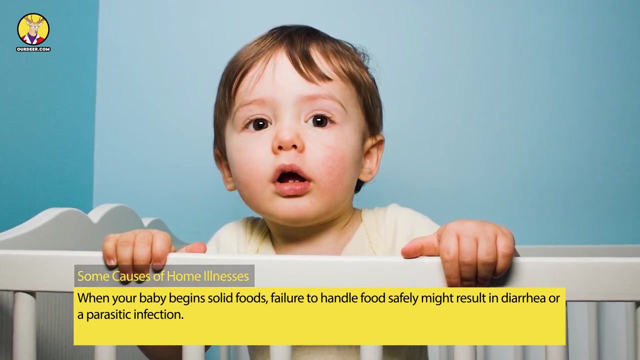 social, social, social education, social causes of home illnesses. Parents should raise babies in healthy home environments, free of allergens and smoke, to prevent respiratory illnesses that can cause developmental delays When your baby begins solid foods. failure to handle food safely might result in diarrhea or a parasitic infection. 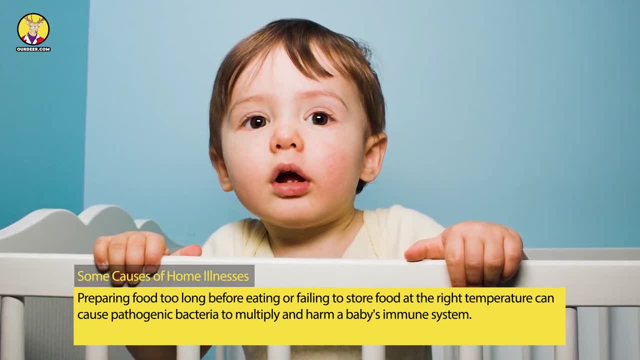 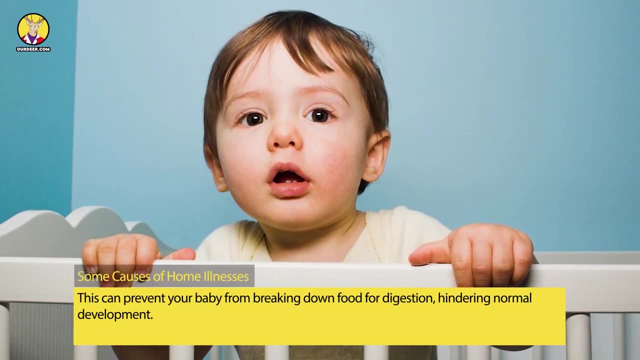 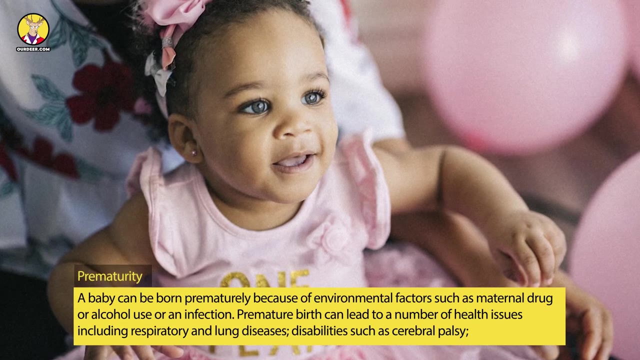 Preparing food too long before eating or failing to store food at the right temperature can cause pathogenic bacteria to multiply and harm a baby's immune system. This can prevent your baby from breaking down food for digestion, hindering normal development. Prematurity: A baby can be born prematurely because of environmental factors such as maternal drug. 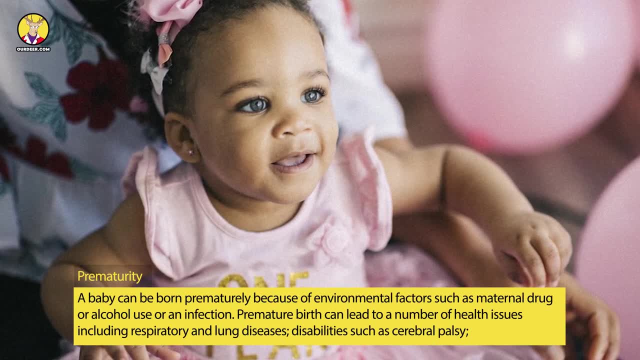 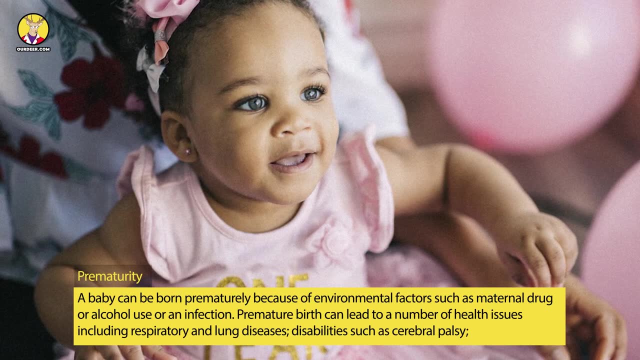 or alcohol use or an infection. Premature birth can lead to a number of health issues, including respiratory and lung diseases, disabilities such as cerebral palsy, bradycardia, a decline in heart rate and retinopathy of prematurity. 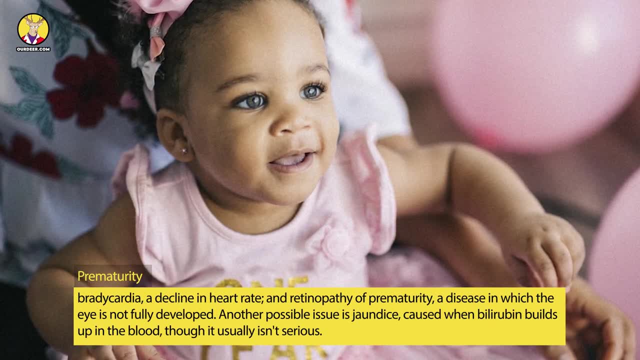 A disease in which the eye is not fully open, can cause premature birth. If your baby is born prematurely, premature birth can lead to a number of health issues that cannot be fully developed. Another possible issue is jaundice caused when bilirubin builds up in the blood, though.